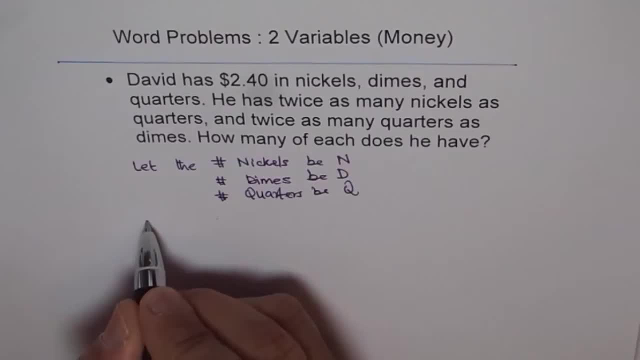 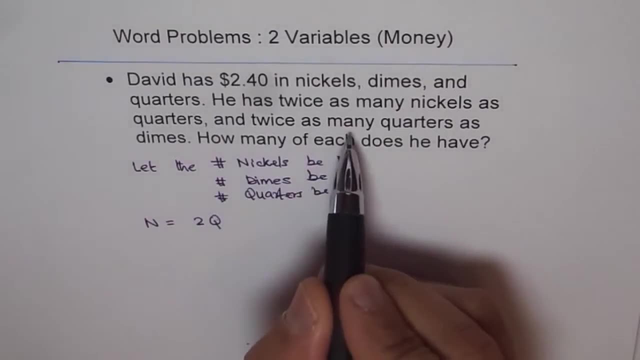 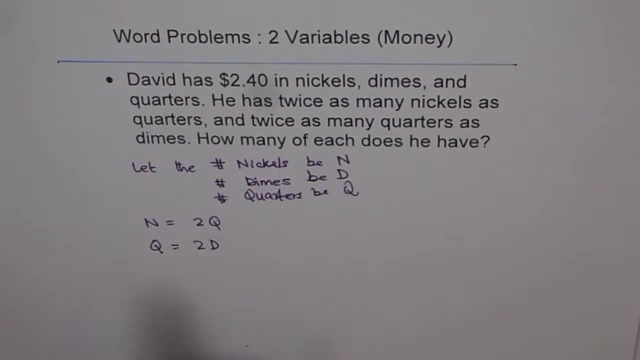 nickels are twice as many quarters. so we have one equation which says: nickels equals to two times quarters and twice as many quarters as dimes. so these are twice times. so we get two equations here. how many of each does he have? that is what we need to find now. let us say he's got all these. 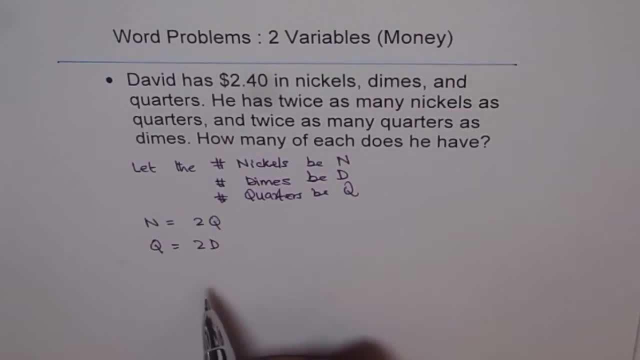 coins. that means the ratio is this. so what is the total amount? when we say that he has two dollars and 40 cents, then this is because of these nickels and quarters. now if there are n nickels, d dimes and q quarters, then how much money will that make? it should make 240, so let's write down this. 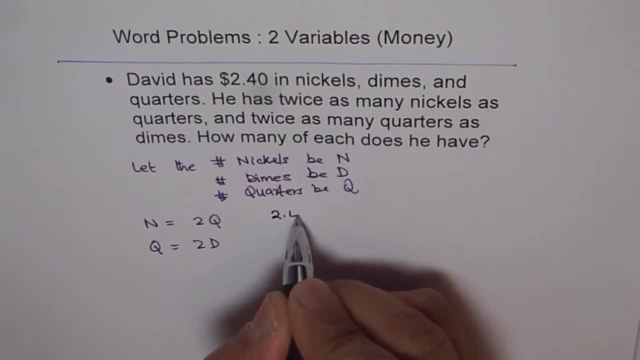 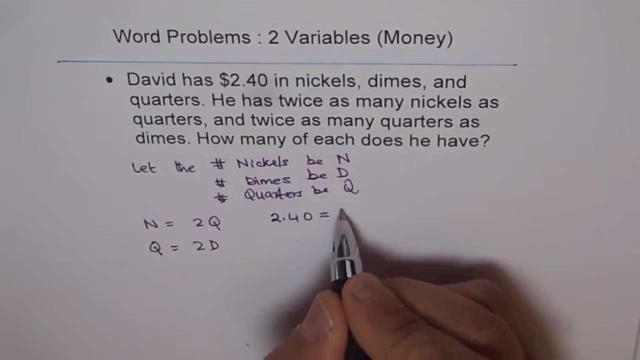 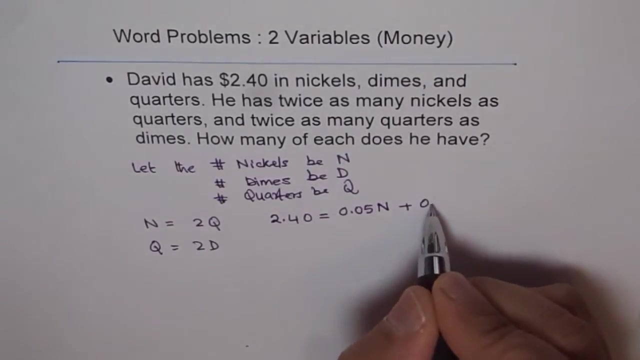 equation, which is two dollars and 40 cents, is equals to: if there are n nickels, value of each nickel is five cents, so it'd be 0.05 times nickels plus dimes is 10 cents, 0.10 times d and quarters is: 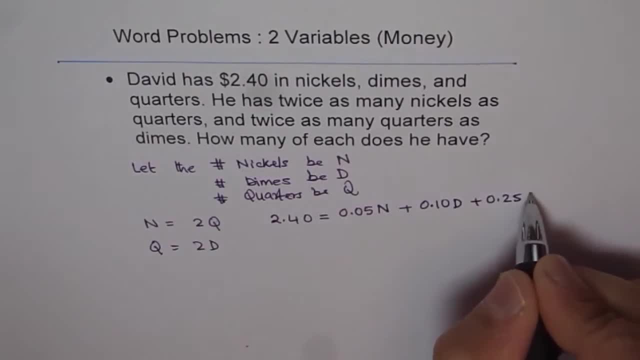 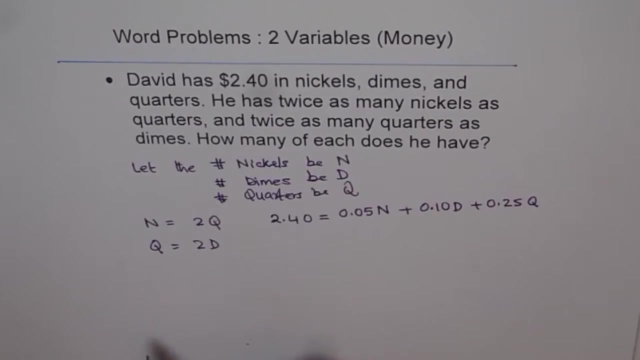 25 cents, 0.25 of quarters. so that is how we get our equation. now there are three variables, just one equation here how to solve it. so best way is to write your variables in terms of one thing. so which one should I choose? nickels is two quarters and quarters is two dimes. well, if I 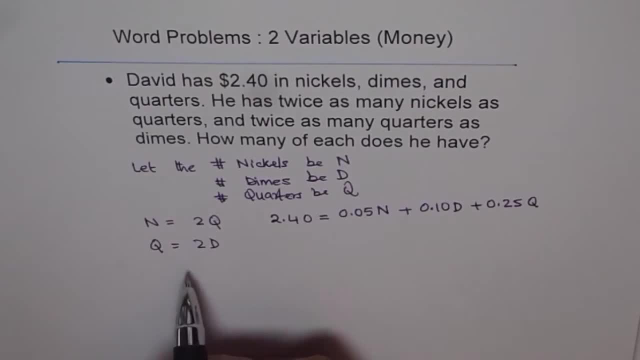 say: nickels is two quarters and quarters is two times, then how many dimes nickel has. let's figure out like that: so nickels has two quarters, quarters is two dimes. so we can write: nickel is equals to two times two dimes, is that okay? that means nickel is four dimes, correct? so we get our. 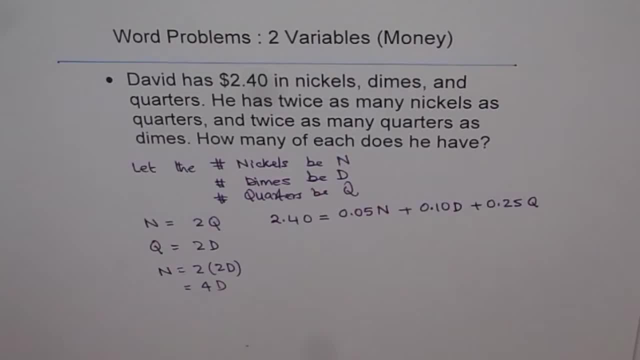 equation where we have everything in terms of dimes. so let's calculate how many dimes we have and then we'll find rest correct, do you understand? so we convert it this side, so we know. now we'll look into these. the quarters are twice the number of times, nickels are four times the number. 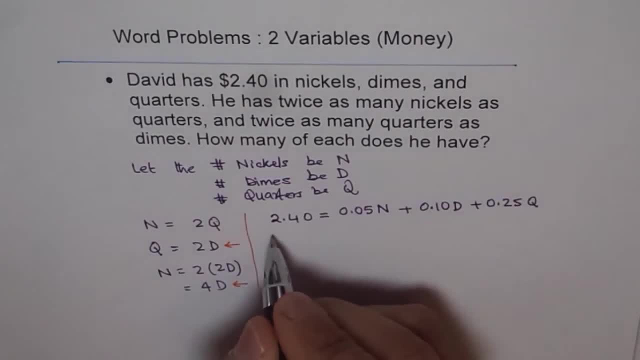 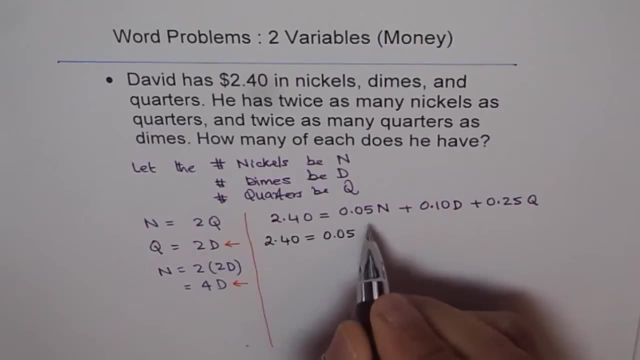 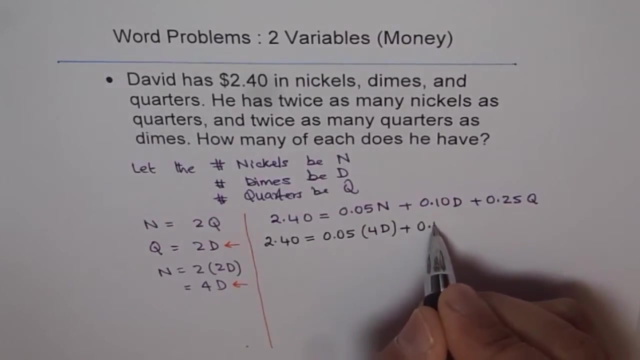 of times. so we'll use this in our equation. so the equation becomes: 2.40 is equal to 0.05. instead of nickels we'll write 4d, four dimes four times right, 4d plus dimes as such, and quarters two times, so 0.05. 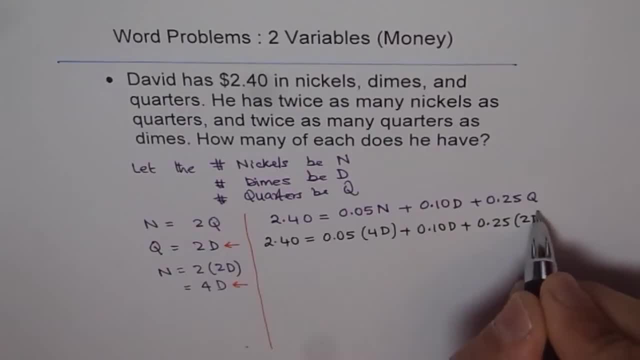 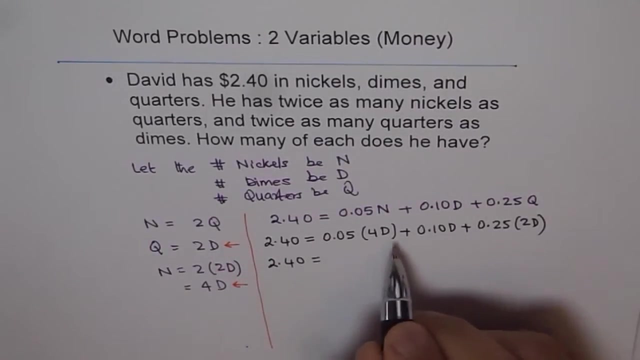 0.25 times 2d. so in this equation we have only one variable, so we can solve it, right? so let's open this up and try to solve it. so you get 2.40 equals to now. dime is common, right? so let me write: and every part has a dime, right? so we'll take dime at the end, or let me multiply. 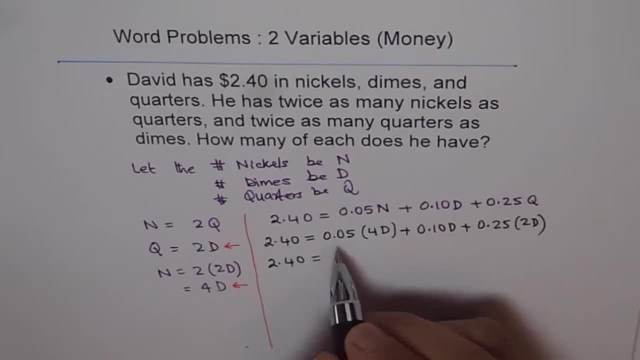 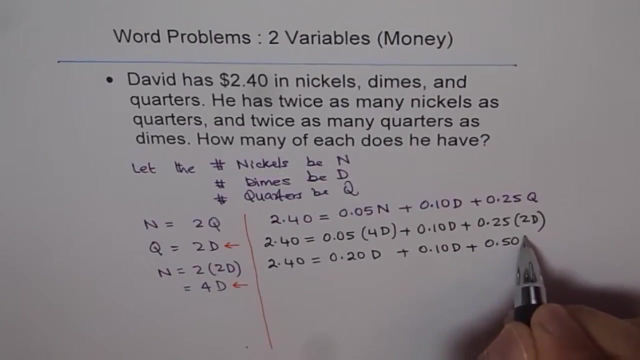 and do it later. so 4 times 5 is 20, so this gets 0.20 dimes, is that okay? so, and this one is 0.10 dimes. plus, if I do two times this, I get 0.50 d right. 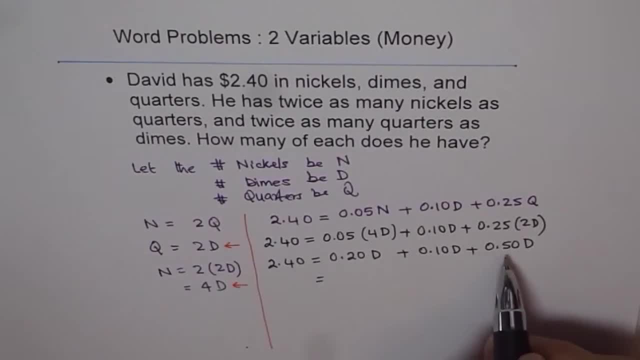 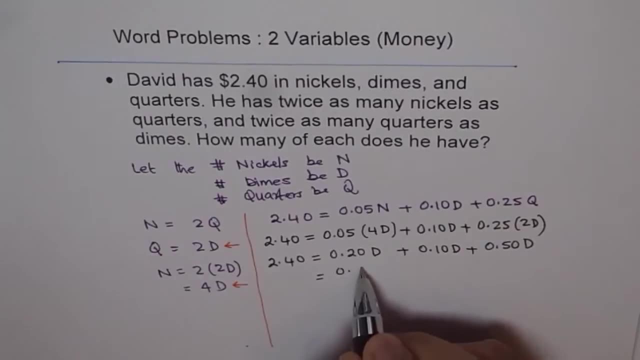 now let's combine all this. so how much do we get? 0.2, 0.1 and 0.5? so 2, 3 and 5, 8, we get 0.80 dimes equals to 2.40. now to find d, we'll divide this by 0.80. 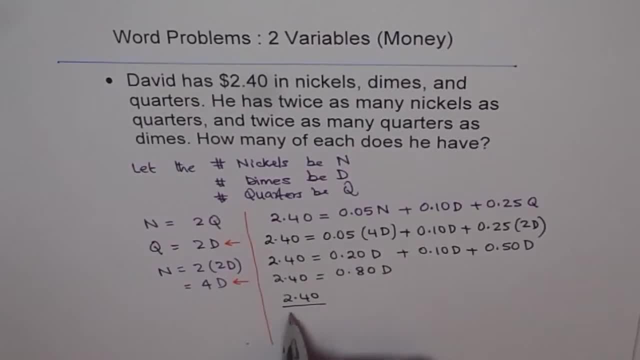 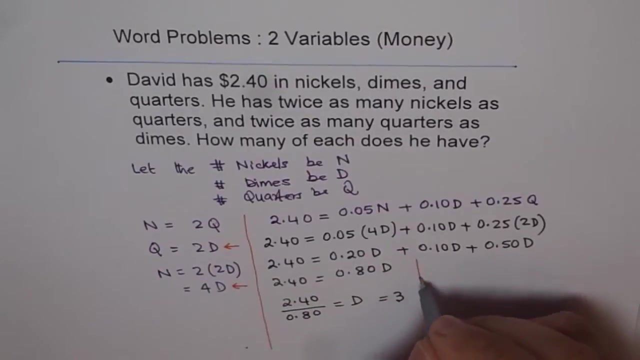 so we get 2.40 divided by 0.80 equals to number of times correct. so what do you get? you can use your calculator, or just 8 is 3 times correct. so dimes is equal to 3. so that is what we get. so we get 3 dimes right now. if we know number of dimes we can write down. 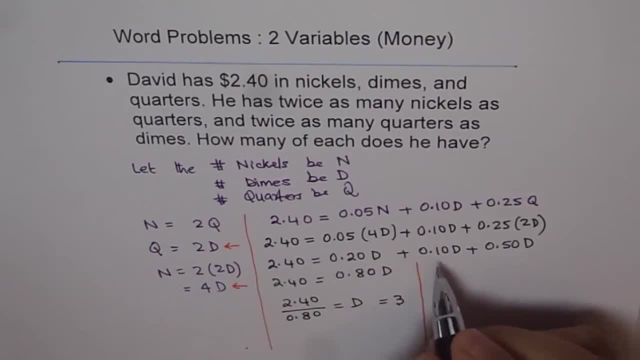 how many are other coins right? so from here we know dimes are equal to t, so that has to be 6 times like. this dimes has a value divided by 1 is equal to d, 2, 9 is equal to 3. now nickel should be 4 times dimes. so nickel. 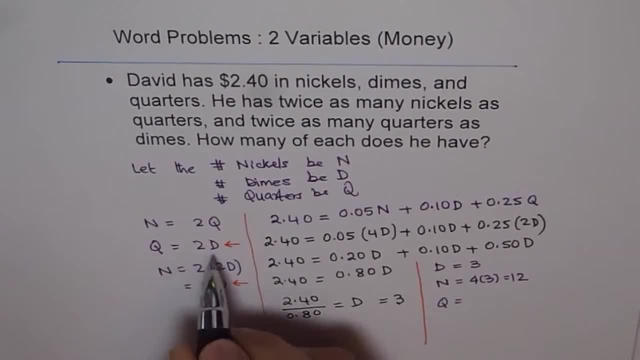 is 4 times times, which is 4 times 3, which is 12, and quarters are 2 times the number of times, so 2 times 3, which is 6, correct? so we can write on our answer now and our answer is that david has.